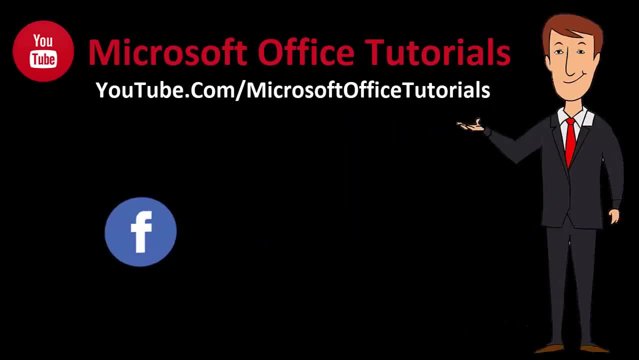 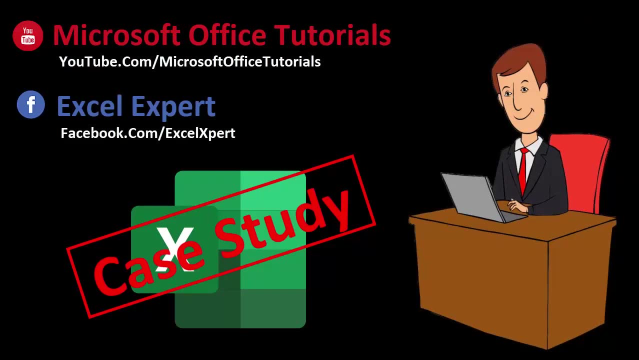 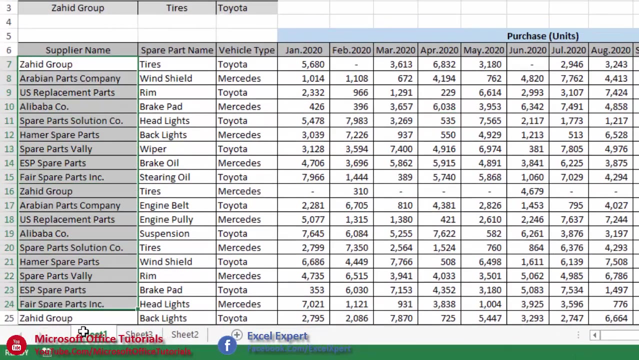 Hey guys, welcome to another video of Microsoft Office tutorials. Friends, in today's video we are going to discuss a case study of Microsoft Excel, or a problem that we need to resolve. Here we have a table in which we have different suppliers from whom we do purchase these different types of spare parts for these. 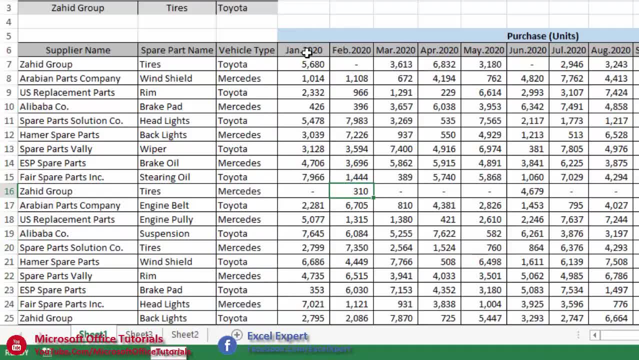 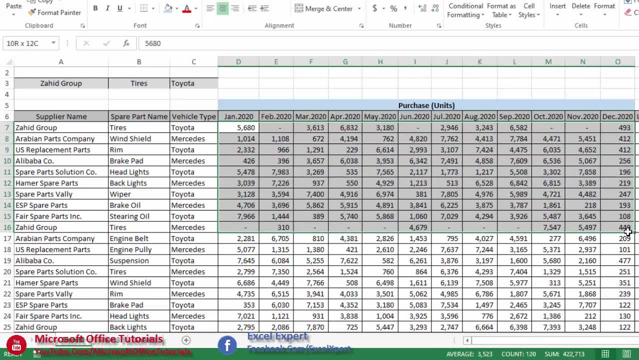 different types of vehicles. Here we have month's name- from January to December 2020- and here we have total units that we purchased during January to December. These units are actually for these spare parts that we purchased for these types of vehicles from these suppliers. Then here we have units sold, and here we have. 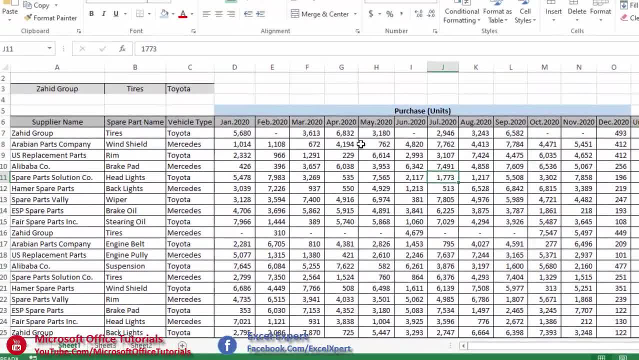 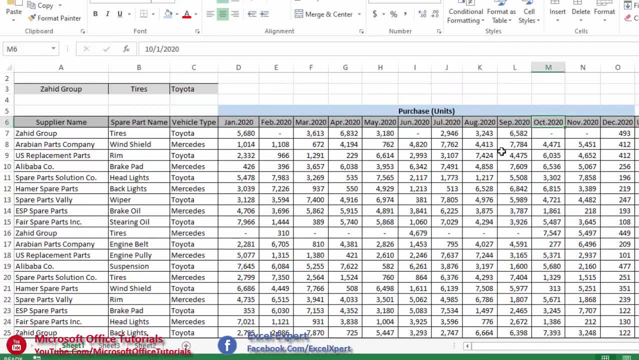 closing balance. Now this is our data or table. Where is the problem? or what is the problem? Actually? the problem is, my manager sent me this sheet and he inserted here three drop-down list. First drop-down list: the suppliers from whom we do. 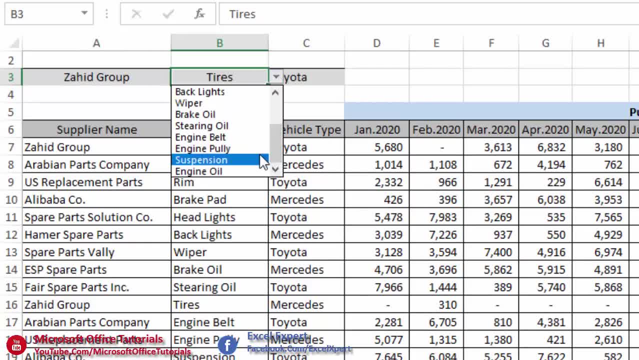 purchase. Second drop-down list: the spare parts that we do purchase from these suppliers. Third, drop-down list: the type of vehicle for which we do purchase spare parts from these suppliers, and my manager want me to insert here a formula or a function that can provide total units purchased from January till. 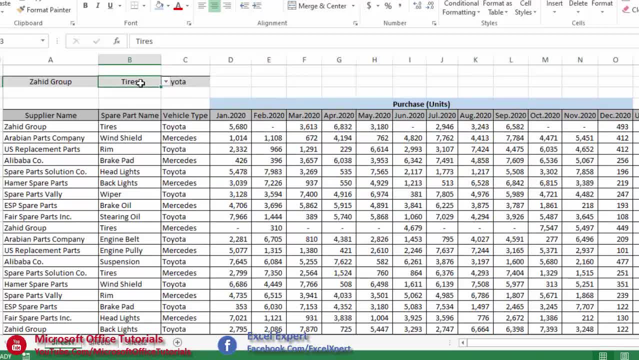 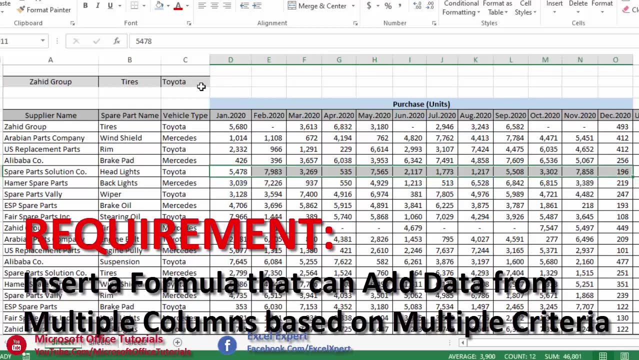 December Units purchased of this spare part for this kind of vehicle purchased from this supplier Indirectly. if we say he want me to insert here a formula that can add these data in multiple columns based on this multiple criteria. So how I can resolve. 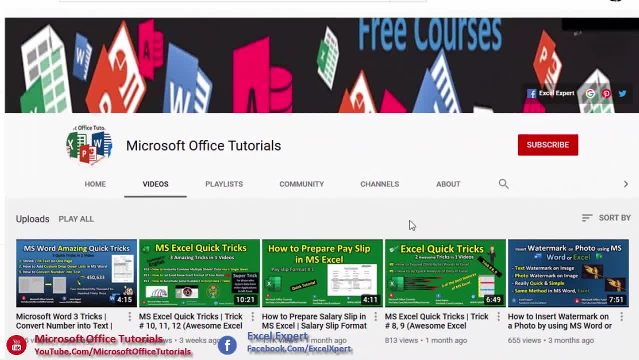 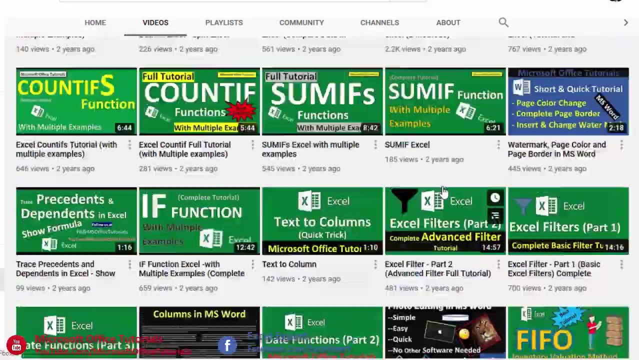 this problem. Friends, before we start the tutorial, if you have not been subscribed our YouTube channel, Microsoft Office tutorials, please subscribe it now And press the bell icon button so that you don't miss any new incoming video. So let's come back to our tutorial. We were discussing that- how we can insert here a 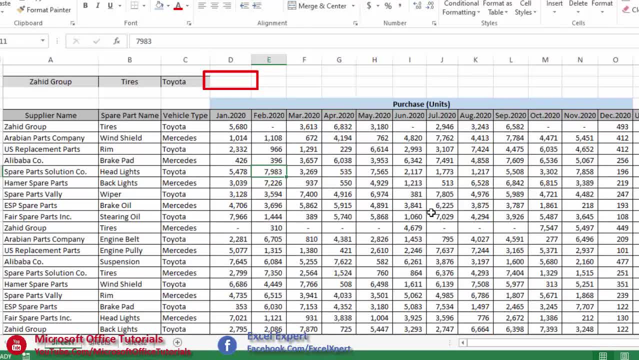 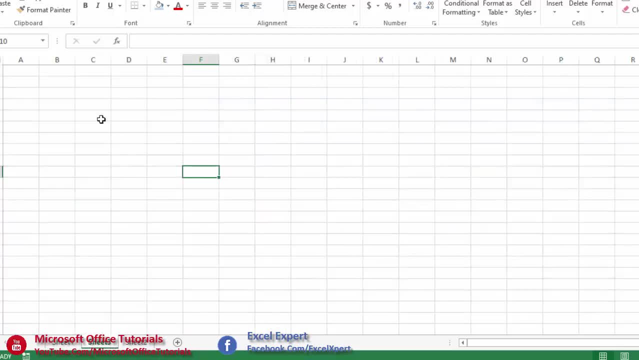 function that can sum or that can add values from multiple columns based on multiple criteria. First of all, when we see this problem, maybe we can think we should use Pivot table. but as we know, if we insert pivot table, it will be inserted in new sheet. 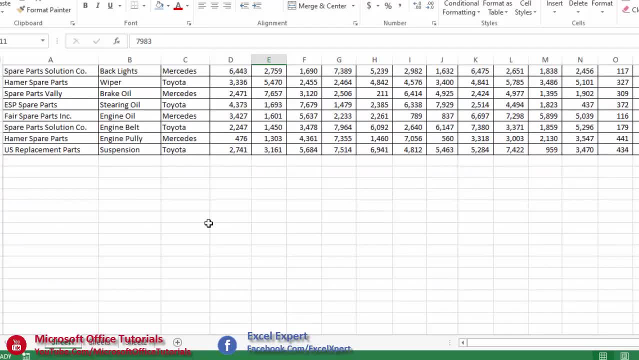 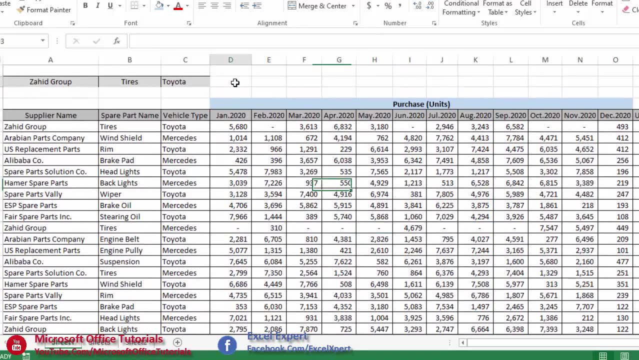 or else where if we insert pivot table on same sheet, it will be inserted below this table. but, as we discussed, manager want us to insert formula here, meaning he want the solution on same sheet in same area in this cell. so using pivot table is not a solution for us. 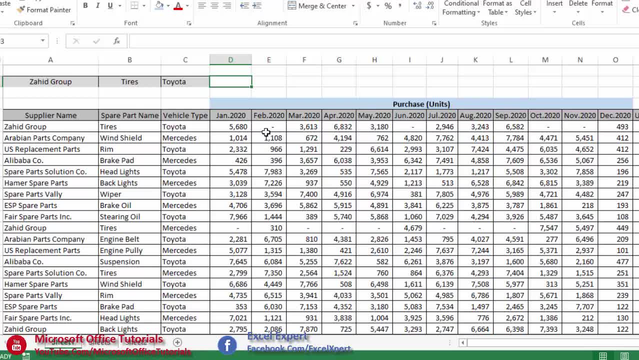 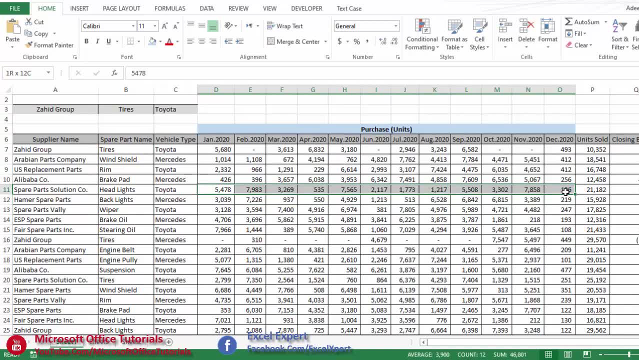 we don't have choice to use pivot table. we have to insert formula here. so we need to create such a formula that can add data in this multiple columns based on this multiple criteria. first of all, let's say we think we should use some if function, because we know in some if function we 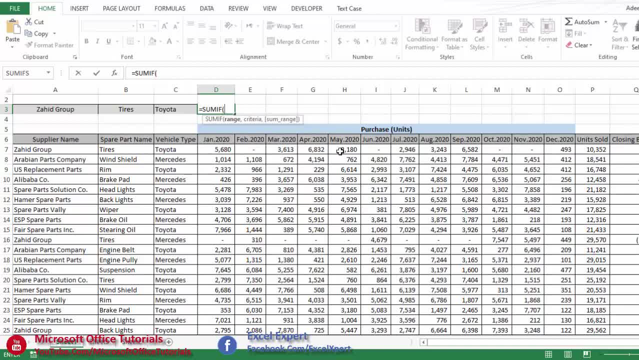 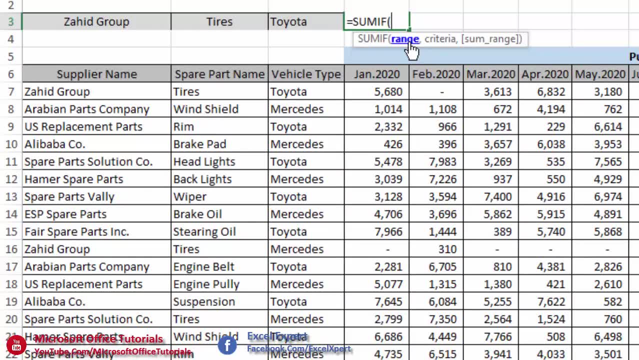 can use criteria and we can use some values, right, so let's try some. if function we have been inserted here from a function and we need to select, first thing that we need to select is range. okay, let's say, this is our first range. these are the 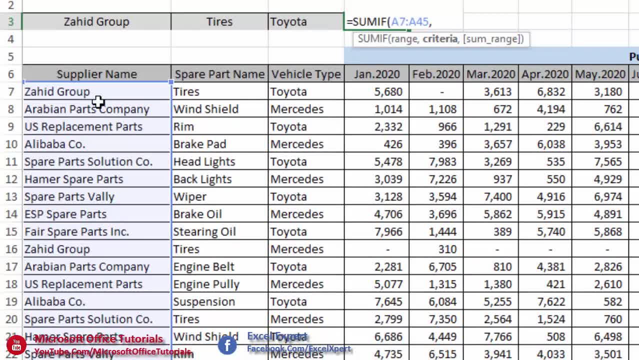 suppliers: comma. in this range. what is our criteria? our criteria is in this cell because any supplier name in the cell. this is our first criteria, then comma and next thing, some range. it is not allowing us to use more than one criteria, as you see. we inserted here first criteria, range. 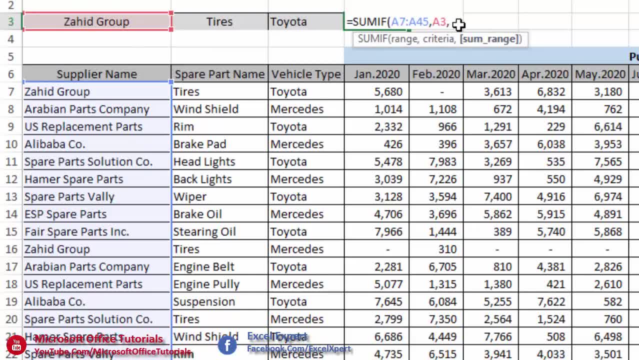 and first criteria and it is not allowing us to insert second criteria, third criteria. so meaning, as we need to use those, they have只有 some number released, and the first is the range. so this means some number is getting reduced or approximately limited, or some number is getting reduced one. 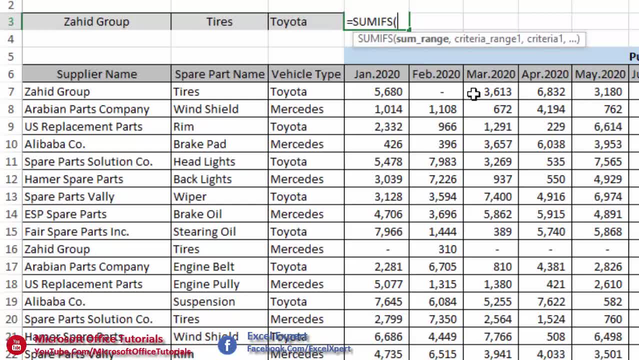 or two high level or they could be limited by two of them like you see some down is limited but I interpret the number to be equivalent for number one so number one this is the number two and will hold back a seven and a half and all the by � North green color is given to be negative 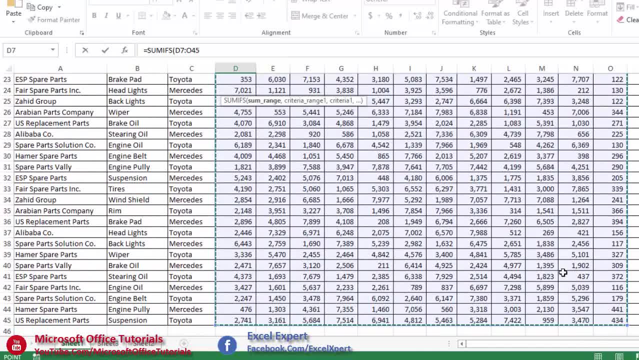 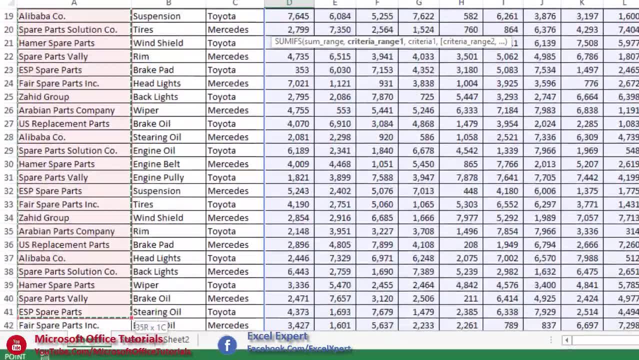 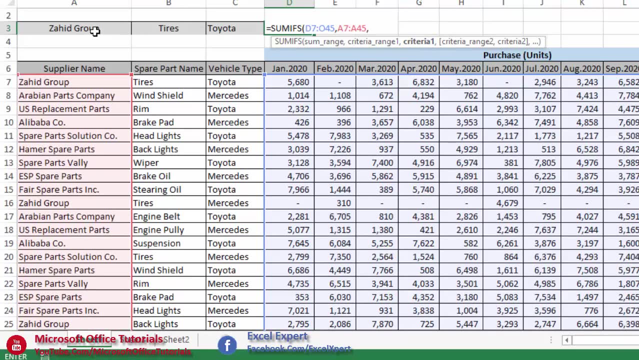 okay, c, this range, this is our sum range, right? so we have been selected our sum range, comma. second thing: criteria range one. this is our criteria range one for our first criteria. this is our range, because our first criteria comma, our first criteria, is this cell in which we have supplier names. so 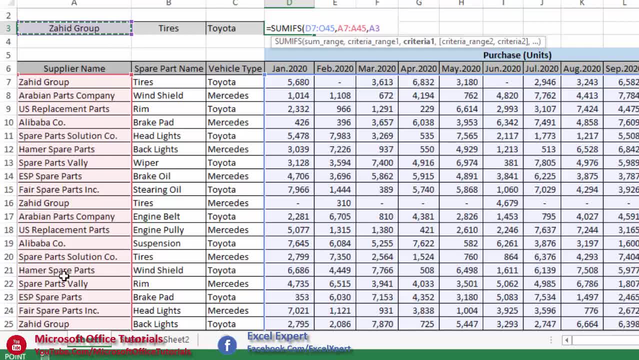 for this criteria? we have this criteria range in which we have all supplier names- comma. second criteria range, this one in which we have spare part names- comma. what is our second criteria? this cell in which we have our spare parts, in this cell, any spare part that we have, this is: 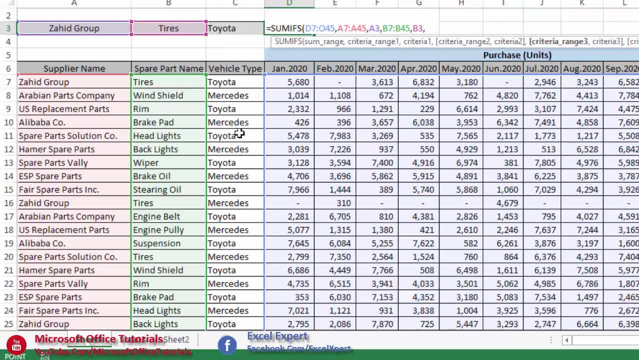 our second criteria: comma. third criteria: range. obviously this column, we select this comma. third criteria: this cell, any vehicle type in this cell. this is our third criteria. so if we have any cut, if this spec lump cut, this is what it looks, the same Hands fixing. so go back, close bracket and seems everything good. right, because here we have been selected. 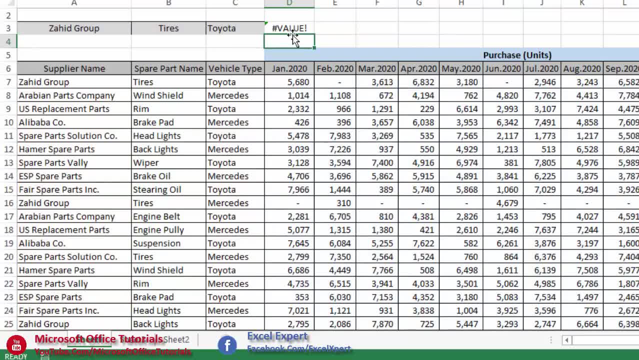 over some range from which we need to add values or units, then criteria and ranges and criteria's- everything we have been selected after Community. and what is this? it is showing us error. why? because if function one column, as we have been selected here, 12 columns, so obviously it will show us our error. 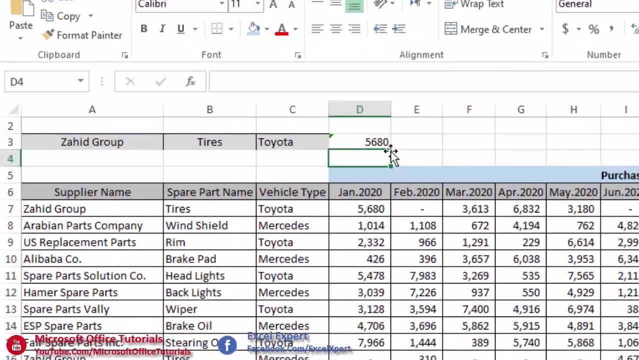 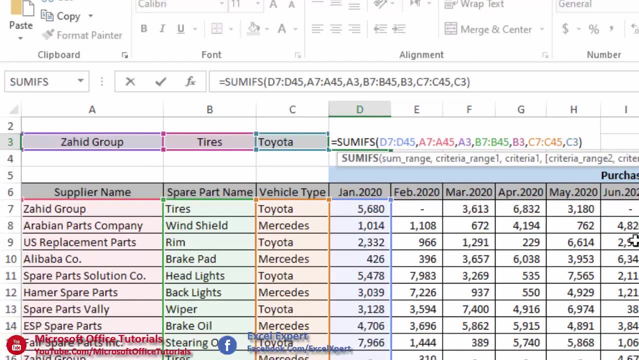 if we select only one column, here we go. it gives us that in january we purchased 5680 tires of toyota from zahid group. but as we know, we need to add multiple columns. if we just let's say we don't add 12 columns, we only add, let's say we say we need january till march, we press enter. it will. 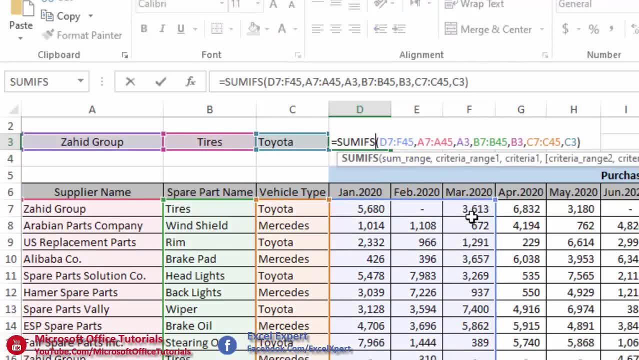 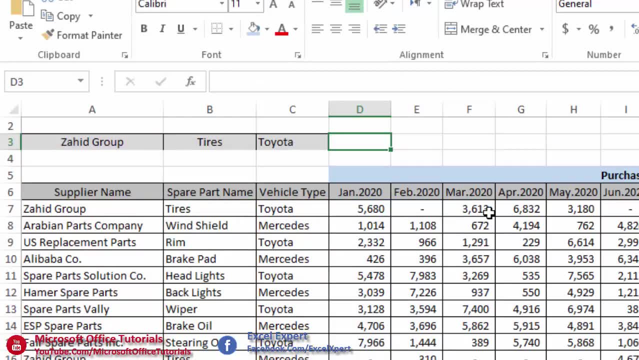 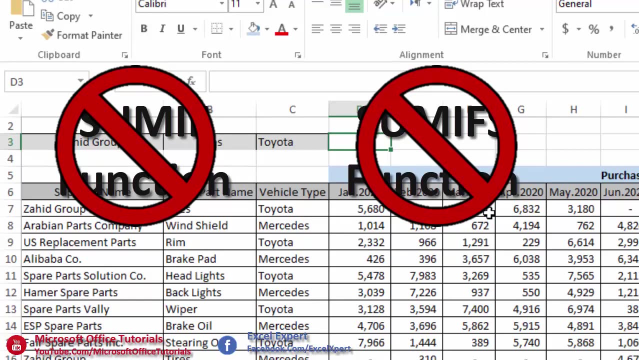 again show us error because, as i said, it don't support more than one column. so this is also useless for us to resolve this problem now. if we cannot use some if function, we cannot use some if s function, then what is the solution? the solution is simple: sum function. yes, we can. 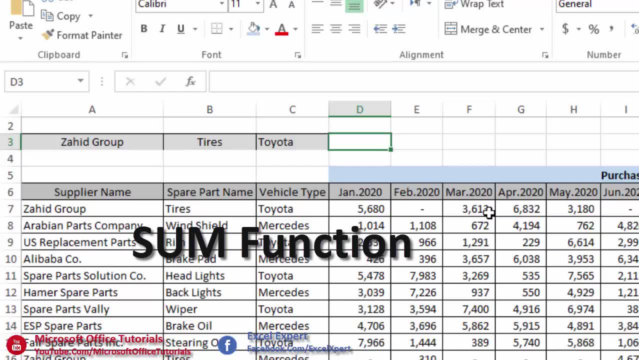 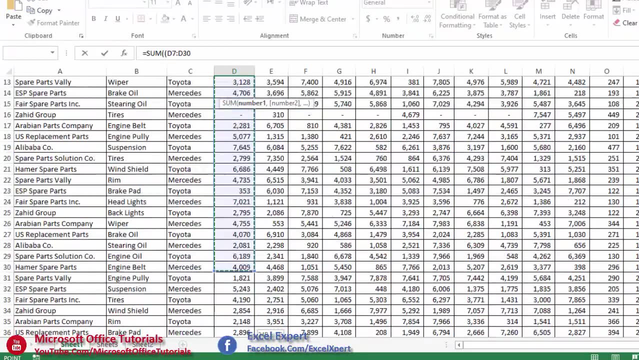 resolve this problem by using simple sum function. so we will simply add here some function. we will insert here one more bracket and as we need to add these, all columns from from january to december, so we will individually select all these columns. the first column for january: we have been selected. 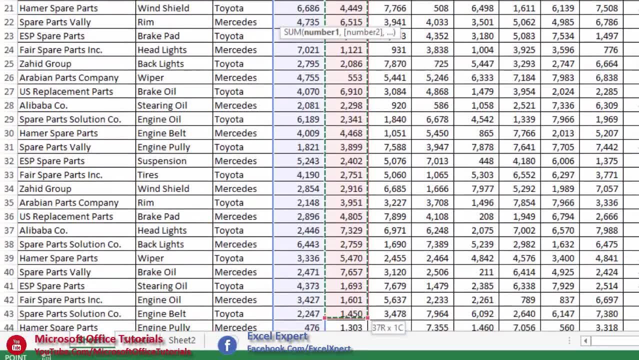 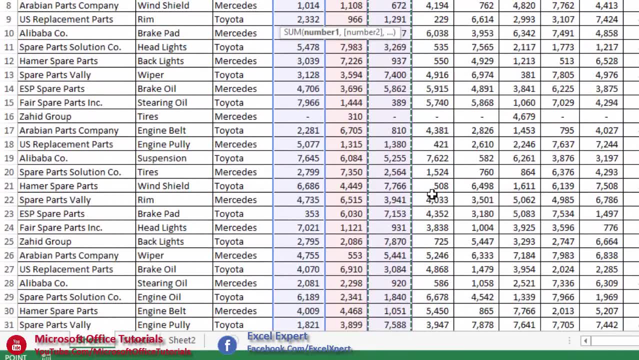 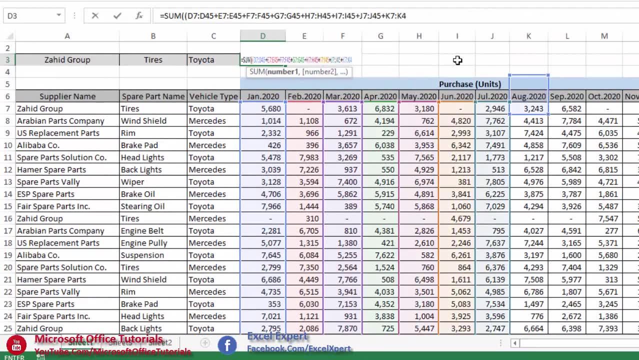 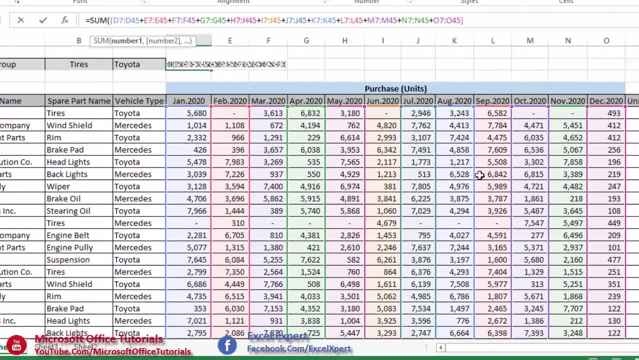 we will insert plus sign. again. for fab, we will select plus sign. for march, we will select this column again, plus sign. similarly, we will select up to december. so i will quickly select all these columns. so, friends, here you can see we have been selected, all columns from which we need to add values. 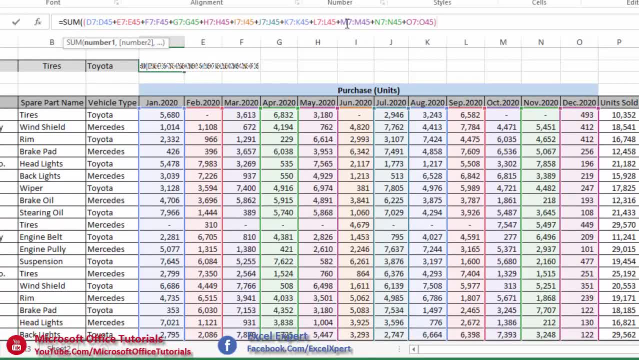 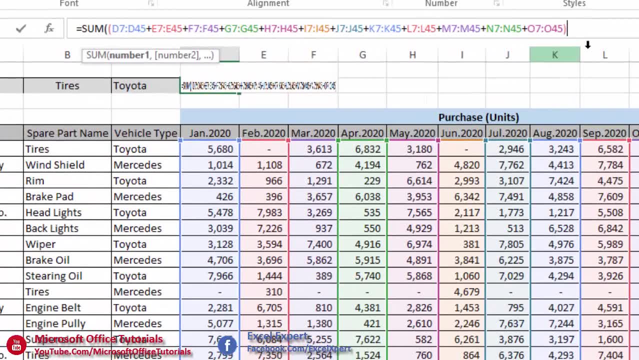 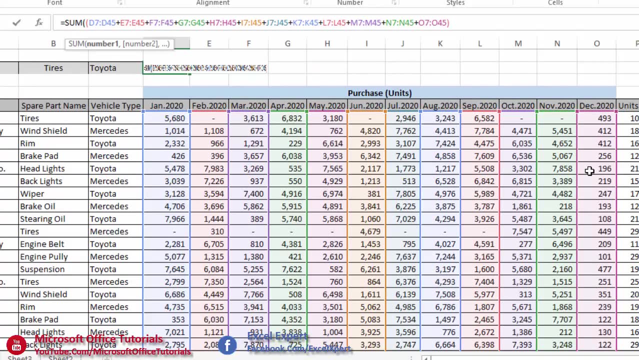 as we need to add values from all of these columns. so we will insert plus sign between the columns and we have been inserted bracket sign because here first part of our formula is complete now as we have been selected all columns from where we need to add values or units. so now we 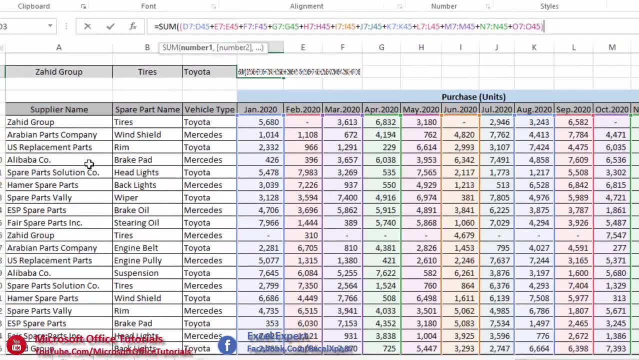 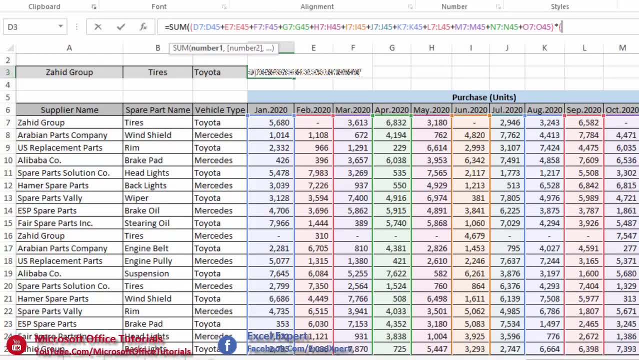 also need to select the criteria or columns based on which we will add these values. now we will insert here multiplication sign bracket. the first criteria range is this column, obviously because our first criteria is supplier name. so in this column we have supplier names. this is our first. 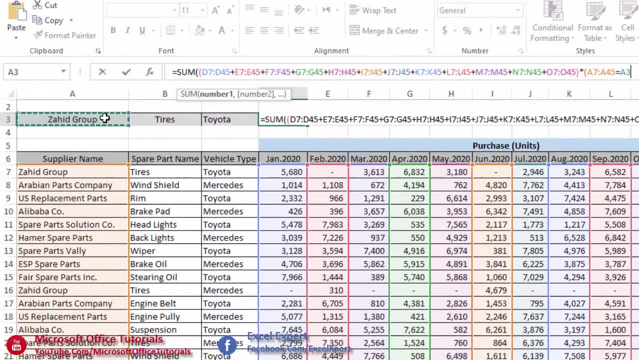 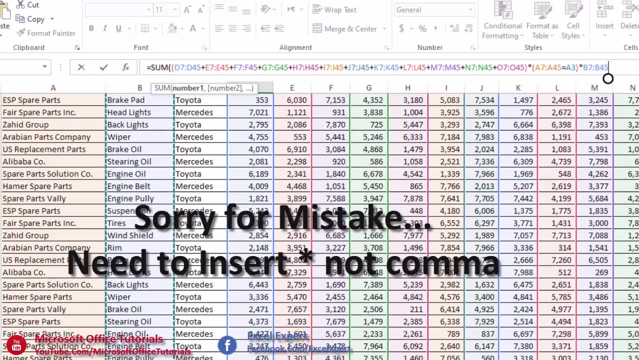 criteria range. this should be equal to this cell because in this cell we have supplier name. any supplier name in the cell should be find here in this range bracket. close again comma for second criteria. this is our criteria range. second criteria range and value in this criteria range. 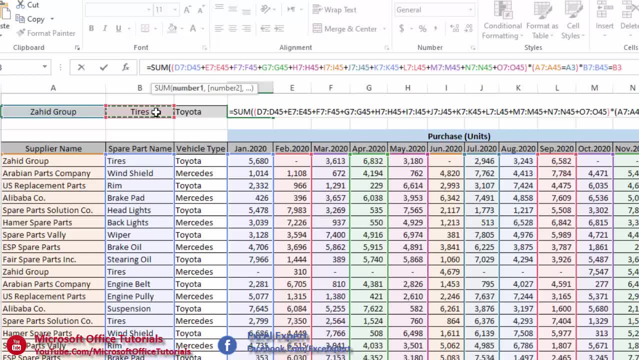 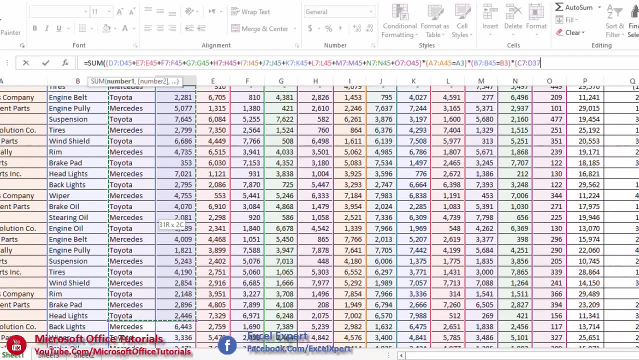 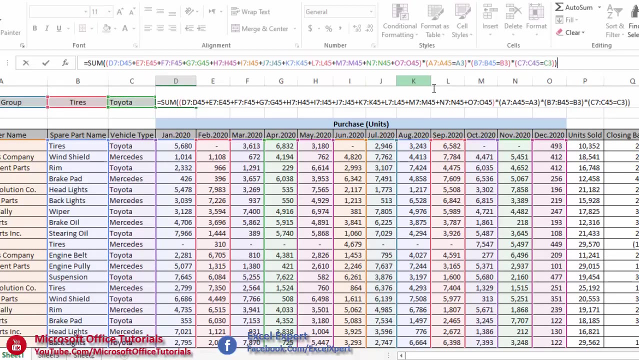 should be equal to this cell. in this cell, any spare part our function should find in this criteria range: bracket close. here we also need to insert bracket actually again, multiplication sign for third criteria. this is our criteria range, obviously, and then equal to this criteria, bracket close. bracket close for function, sum function. and now, as you can, 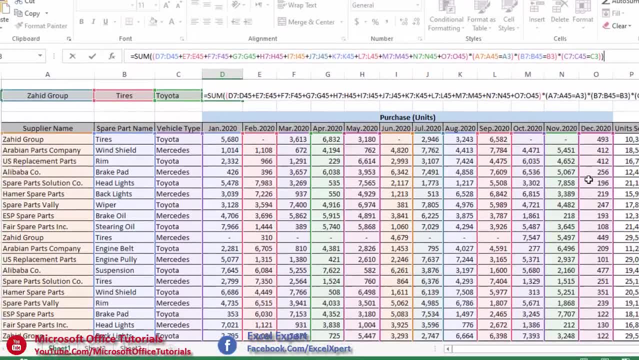 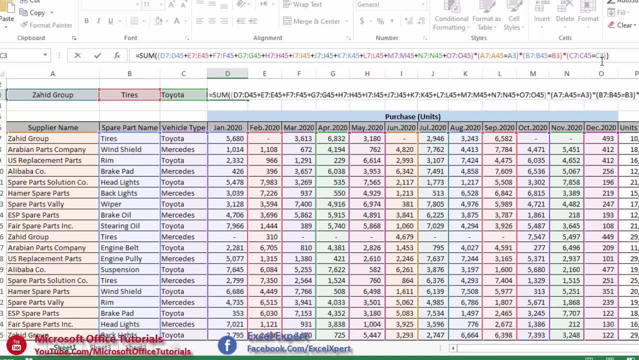 see, we have been selected all columns from where we need to add values. then we have been selected all criteria ranges from which we need to select all this criteria. right now. one more thing we need to do: we need to insert one more bracket with each of this criteria range and criteria, and out of this bracket we 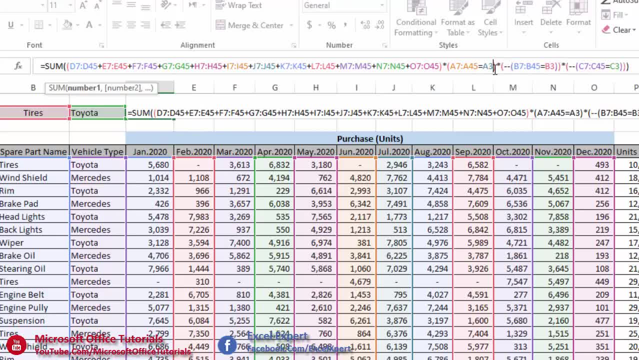 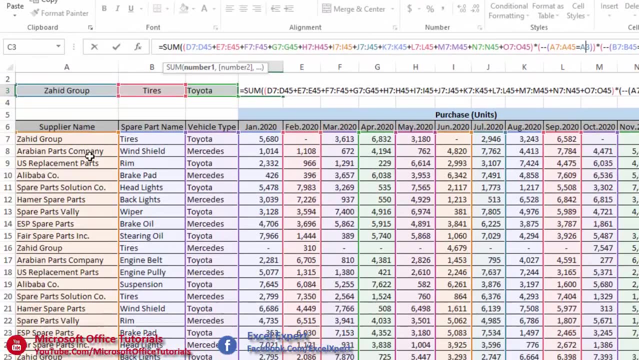 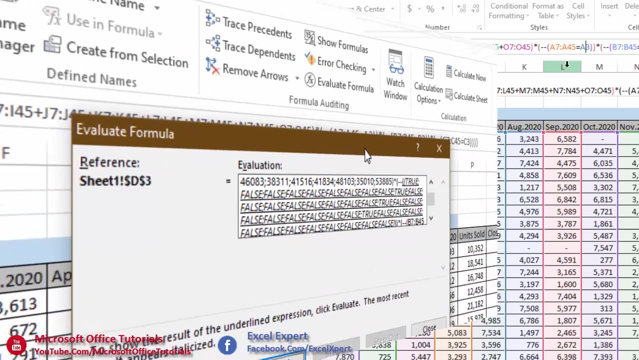 need to insert two times minus sign. now the question is why we inserted this sign two times with each criteria, range and criteria, because these parts of formula, each of these, will try to find this criteria from each of these cells and if we it will find the criteria in any of these cells, it will give result in form of true. 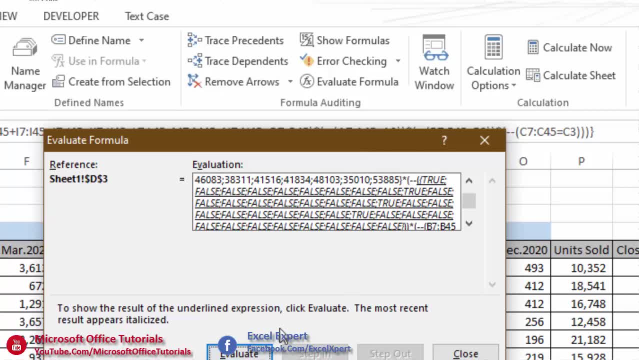 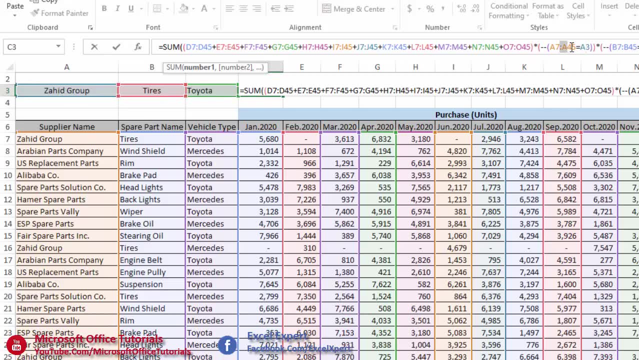 and if it will not find the criteria, it will give result in form of false. for example, for this first criteria, zahid tractor, this part of formula will try to find zahid group in all of these cells. if it will say find zahid group in first cell, it will give result as true. in second cell it will not. 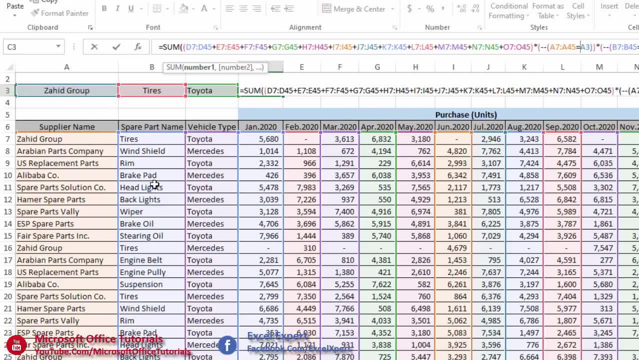 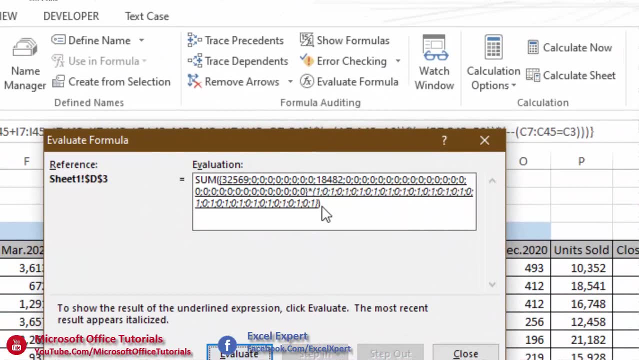 find zahid group, it will give result as false and so on. and when these all of these three parts will give result for each of these cells as true and false, this minus sign will convert true and false into one and zero. this minus sign, these two minus signs, will convert true into number one and false. 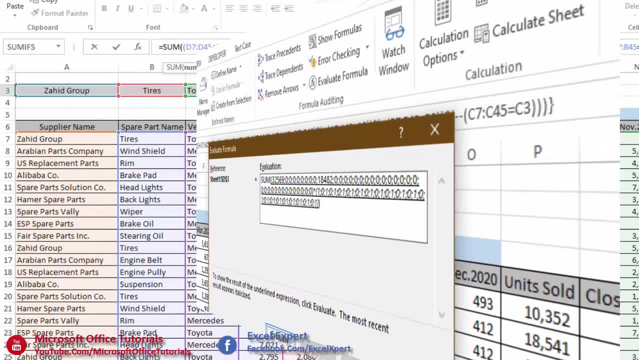 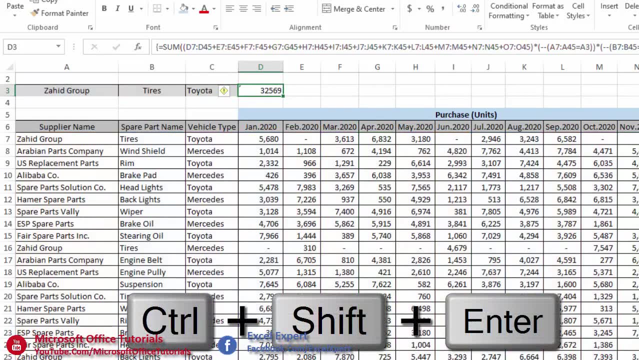 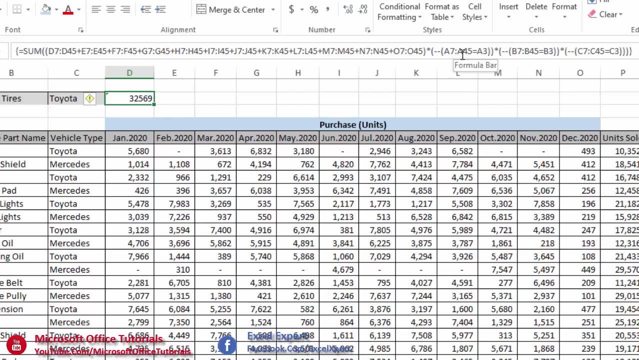 into zero. now, the last thing that we need to do to complete our this formula, we need to press ctrl plus shift plus enter button. when we will press, you will notice here curly brackets with this function. this curly bracket shows that our formula is converted into array formula. 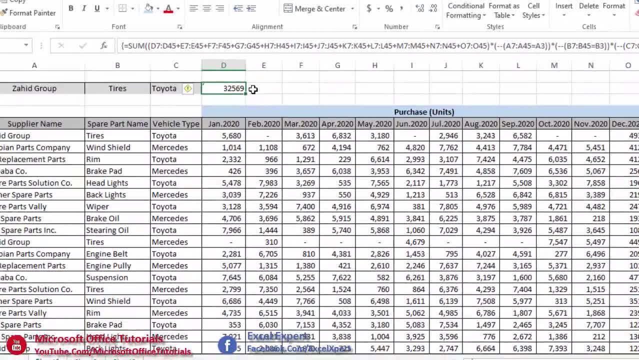 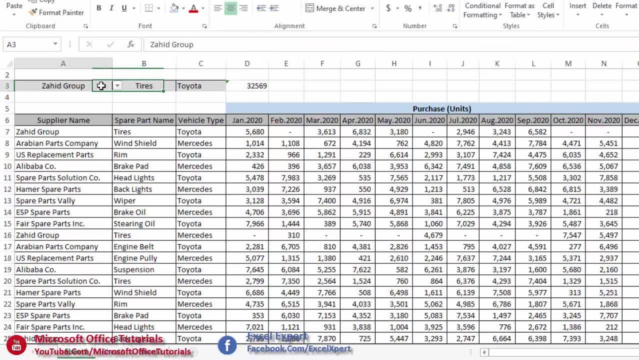 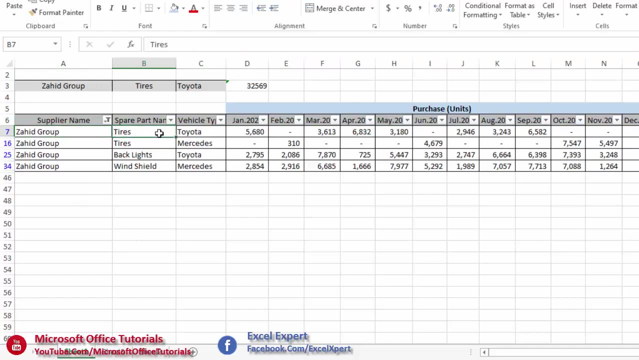 and if you see the result, this is showing us that we purchased for toyota. we purchased 32 569 tires from zahid group from january till december. let's check this formula, cross check this formula, we will insert filter and we will filter supplier as zahid and from zahid. we purchased tires for toyota from. 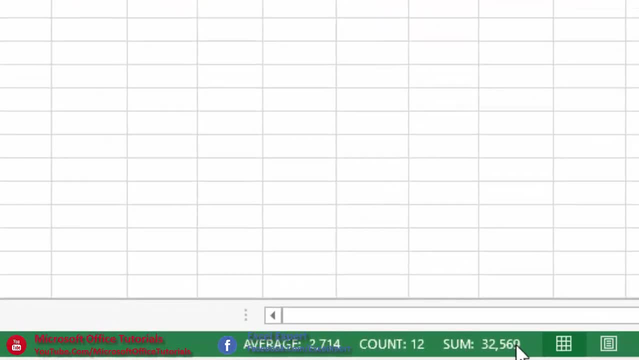 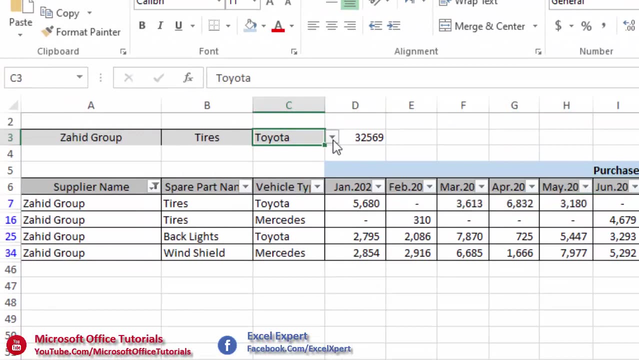 january till december. if we select this is 32 569, exactly the same. that is result of our formula. let's try something else. we change vehicle type from toyota to mercedes. shows that we purchased 18 482 tires for mercedes from zahid tractor from january till december.